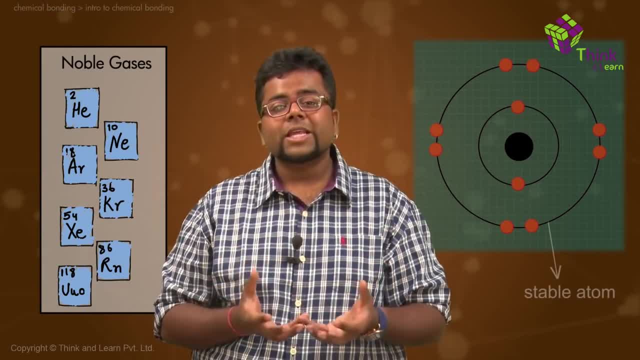 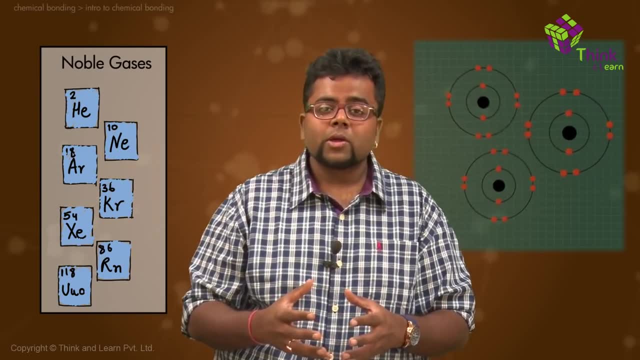 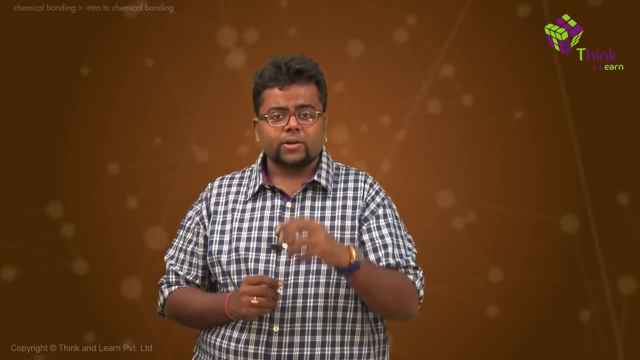 And we know that the noble gases are the most stable atoms or the most stable elements for us, Because they themselves do not want to form bonds with their own species. Right Now, this completion of octet is what is called as the octet rule. 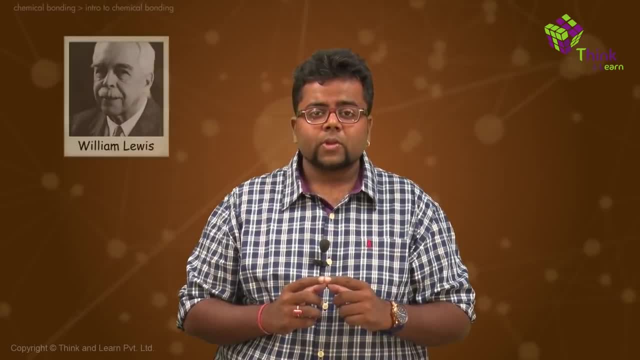 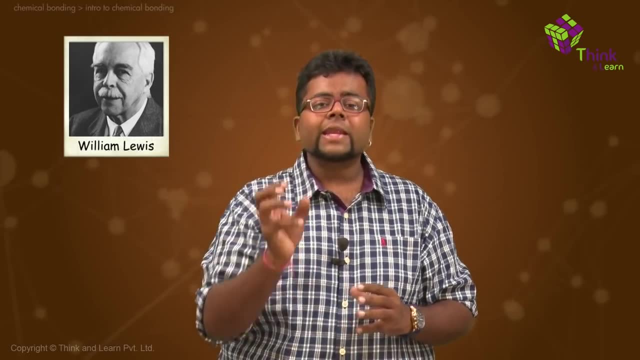 Now there was a scientist called as Lewis. What he did was he tried to show that how does an atom look like? or how would we represent an atom while forming bonds? Because we cannot show all the electrons, the neutrons, protons and everything. 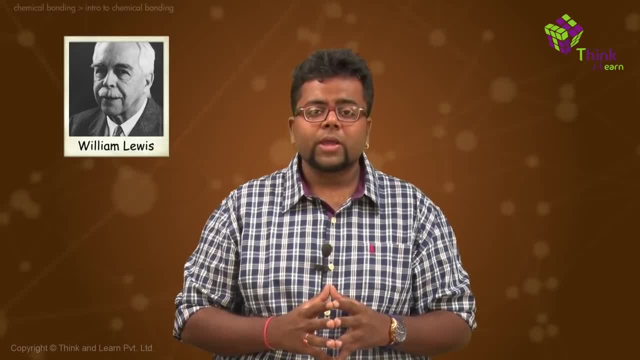 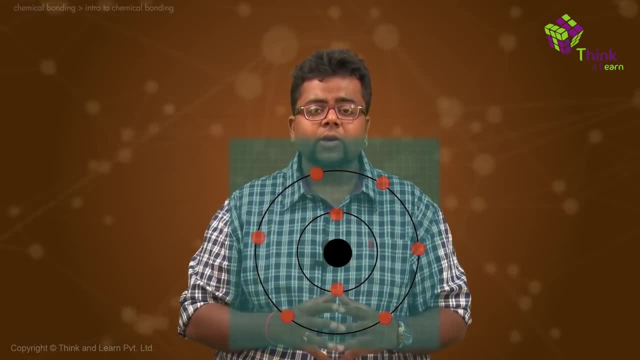 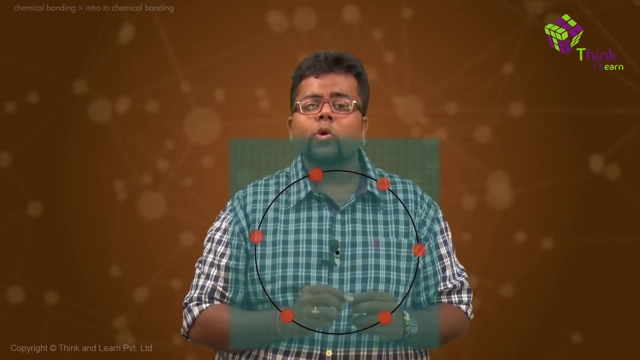 because that would make the things more stable, Complicated. So what he tried to do was he tried to simplify everything. So he said, except the valence shell electrons, everything else will take it as a small point and that point would have a positive charge. 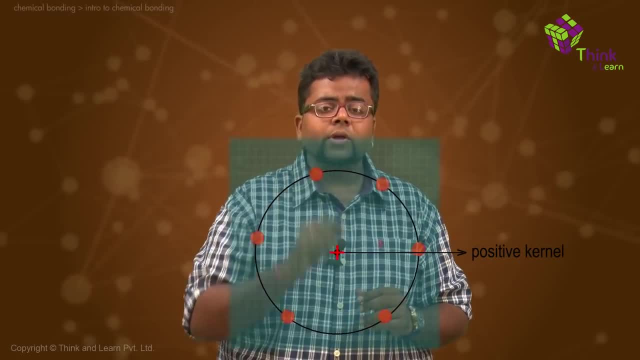 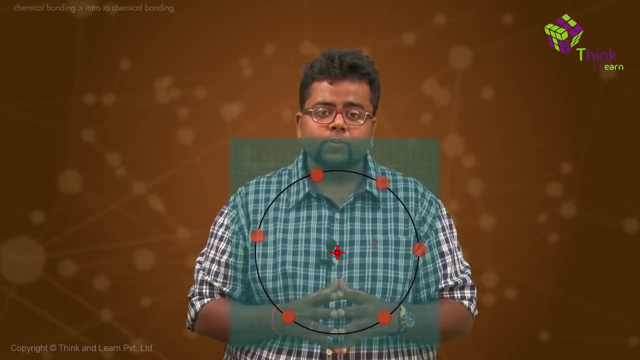 and would be called as a positive canal. Now, why the term positive? Now for an atom. we know that the number of protons and the number of electrons are equal. Now, if I only consider the inertial electrons and the protons, 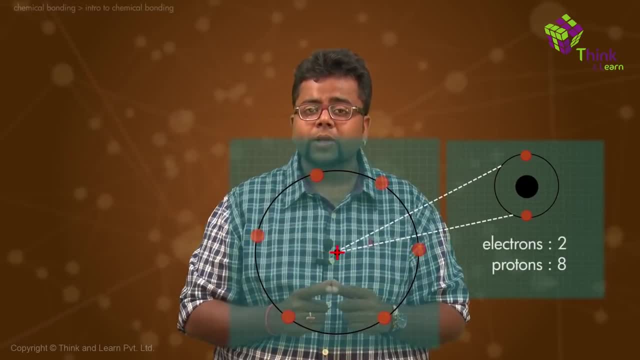 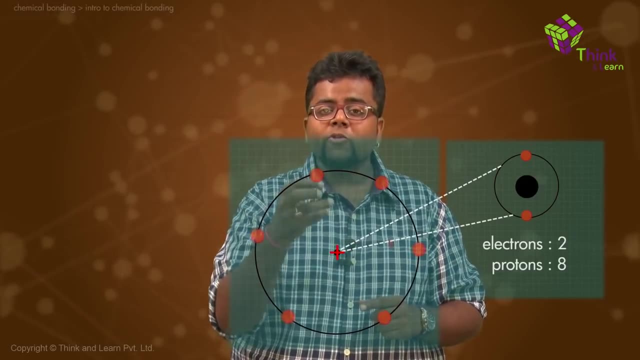 the ratio in which the protons and electrons are present, the number of protons would be higher. So that means in that entity you would have more of positive charge. That is why the charge positive And by the English word canal. 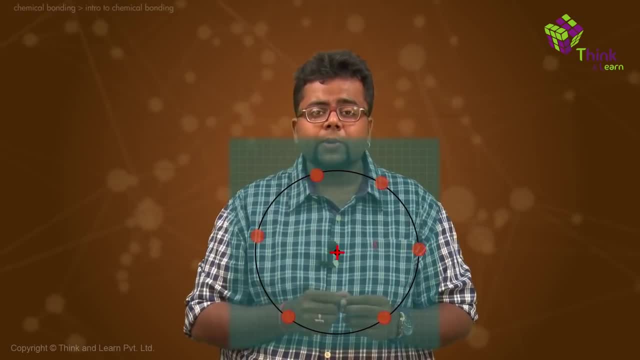 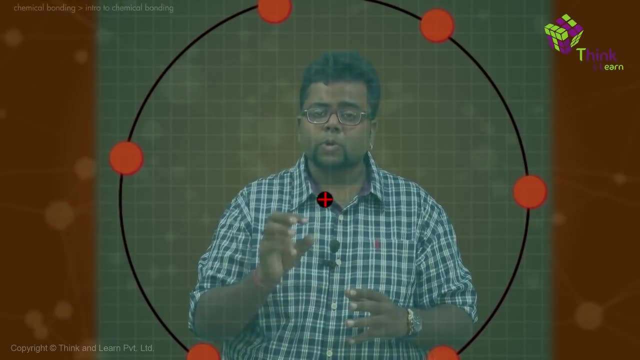 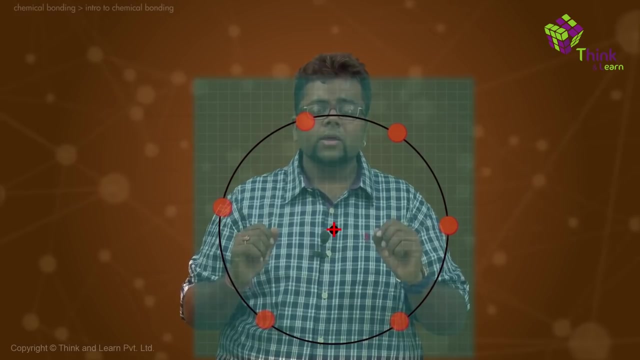 means a very small crystal or a very small, tiny particle. That is what is called as canal. So that is why this entire thing comes to be known as a positive canal, And the valence shell electrons are left as it is. So this is the complete representation of an atom. 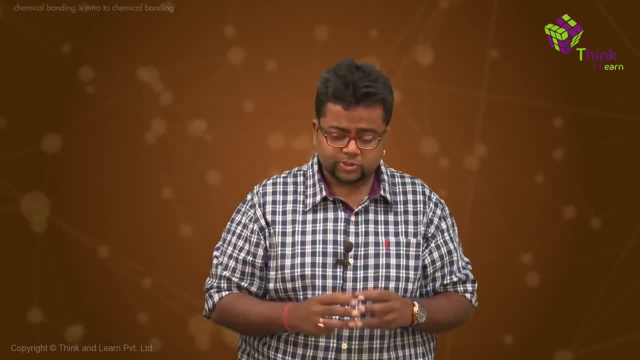 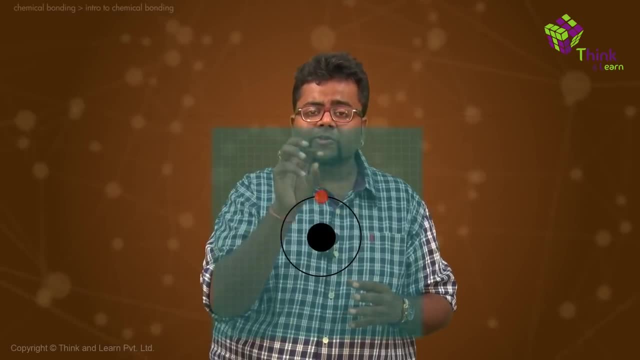 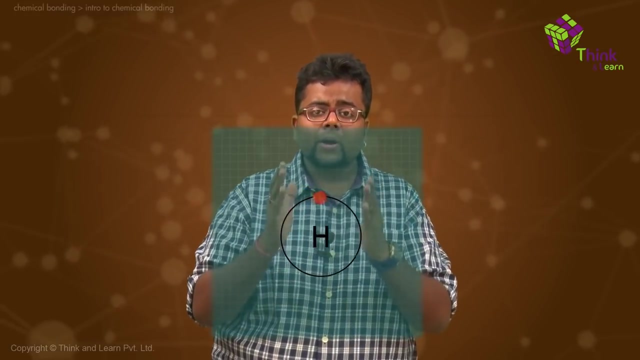 Now if we take different atoms, suppose if I take hydrogen Now, hydrogen would not have any inertial electrons. So what happens? The positive canal would only be that one proton that is there, and we will represent that positive canal by the symbol itself. 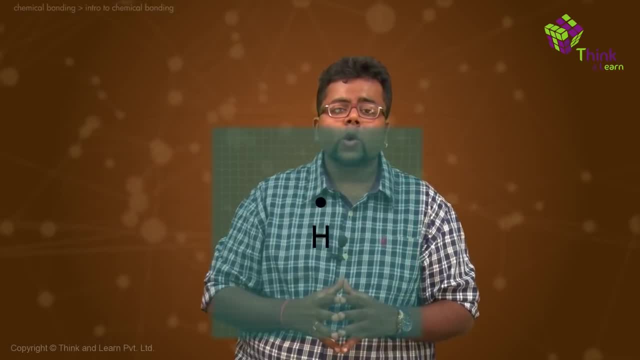 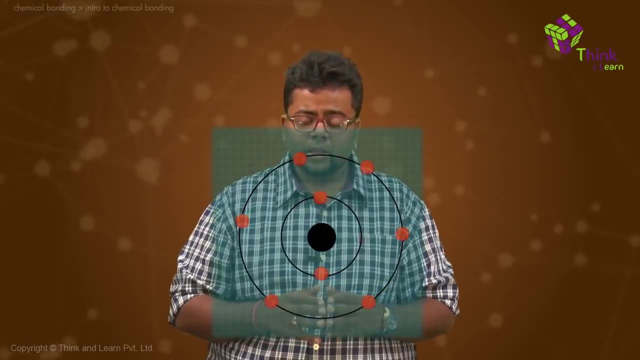 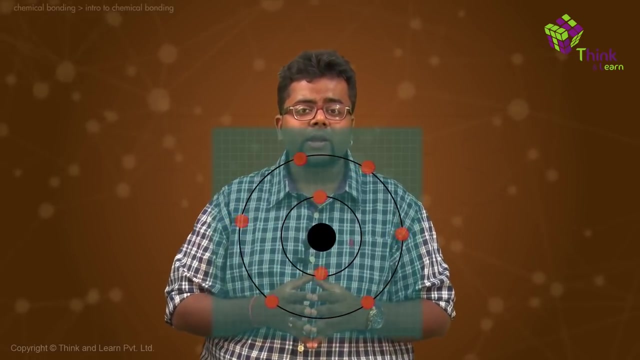 So we will write it as H And we will put this dot over here, which is representing that one valence electron that hydrogen has. Now let us take oxygen. The total number of electrons that the oxygen has is 8. And the general electronic configuration that we write is 2, 6.. 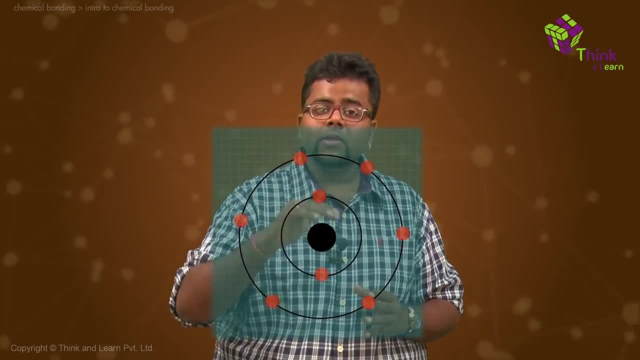 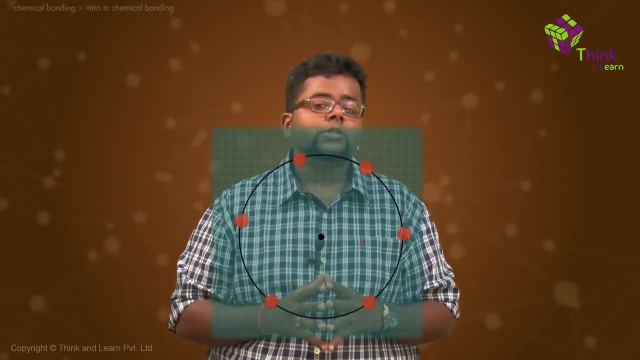 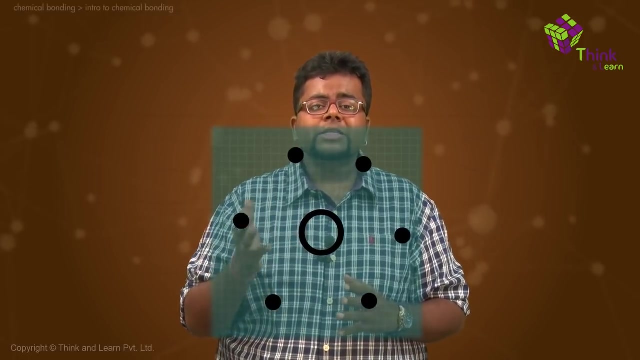 So that means 2 electrons are present in the inertial and 6 electrons are present in the outermost shell. So how would the Lewis structure for oxygen look like? So you will have O, which is representing the positive canal, and we will mark 6 dots. 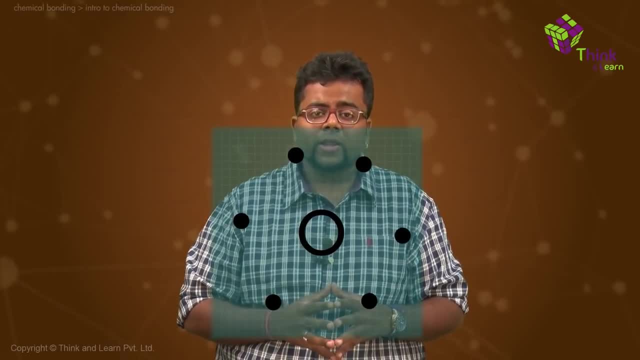 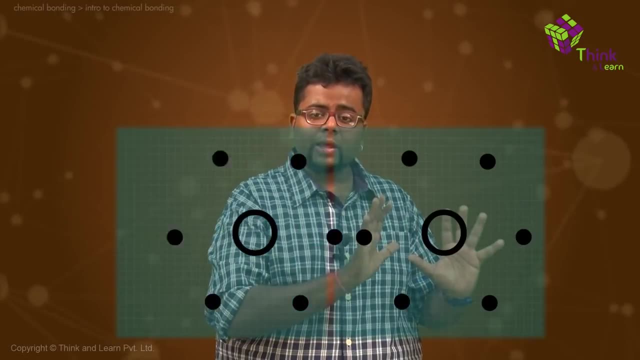 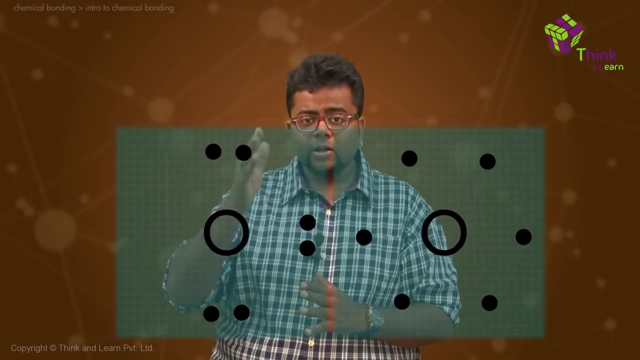 All the 6 dots representing an electron H. Now you just cannot have the placement of these dots randomly. I cannot represent a Lewis structure of oxygen like this. It has to be symmetrical, where I can draw a plus 2 electrons on this side. 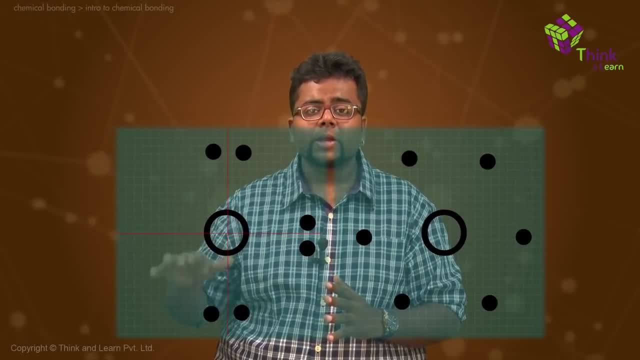 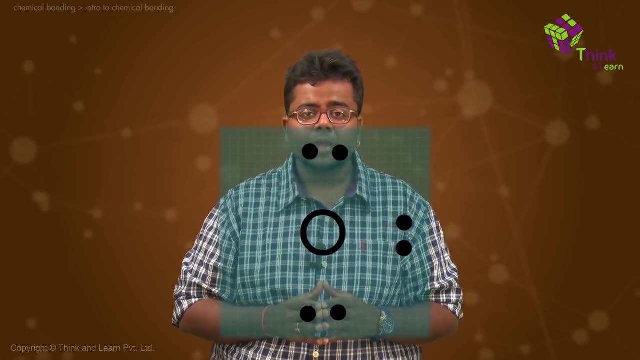 2 on this side and 2 on this side, So this side would be completely empty. So this is how a symmetrical representation of Lewis structure is done. Now let us talk about, say, nitrogen. Now for nitrogen again. 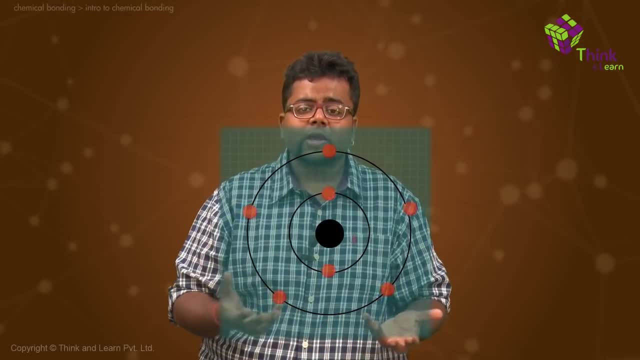 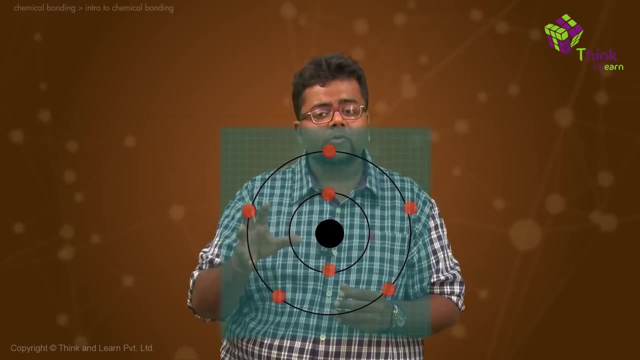 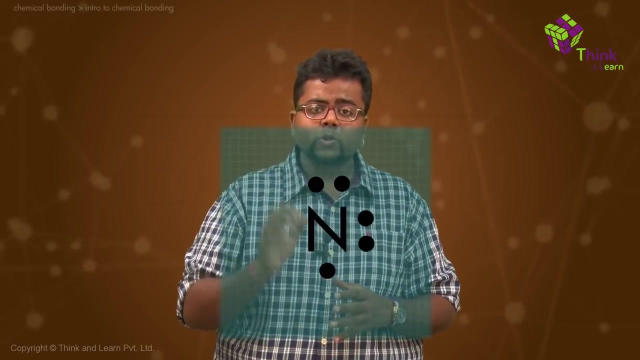 we would have 5 as the electronic configuration, because it has 7 electrons in total. So the 2 electrons would become part of the positive canal And that representation would become N, And the 5 electrons that we have would be 2, 2 and 1.. 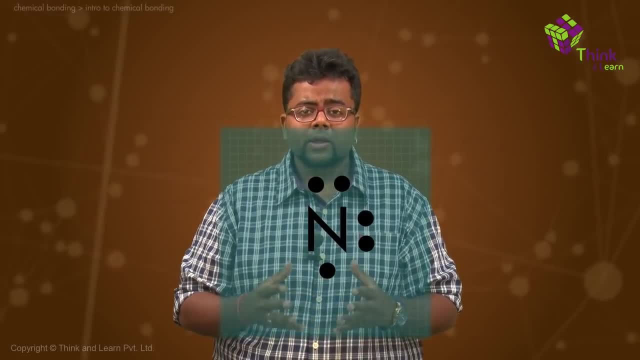 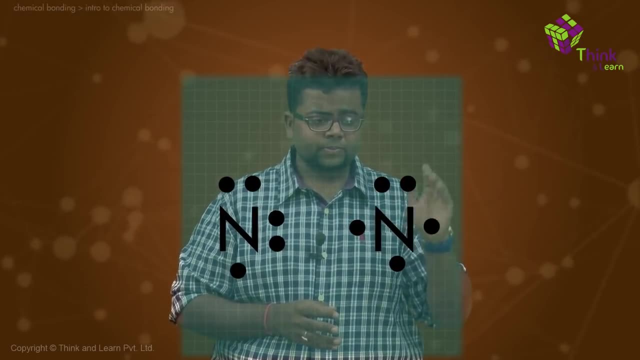 So that is how the nitrogen can be represented. Now in some books they also represent nitrogen as N, 2 dots: 1 dot on this side, the other one on this side and 1 at the bottom. So what they are trying to do is: 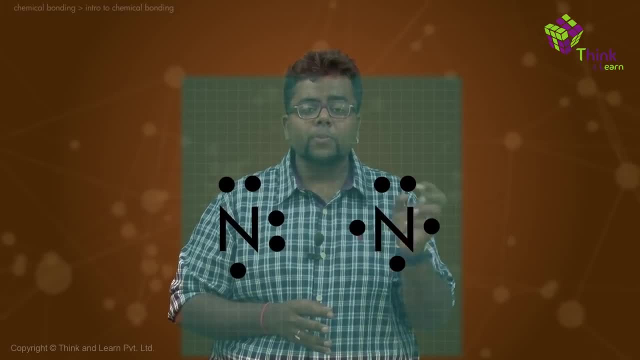 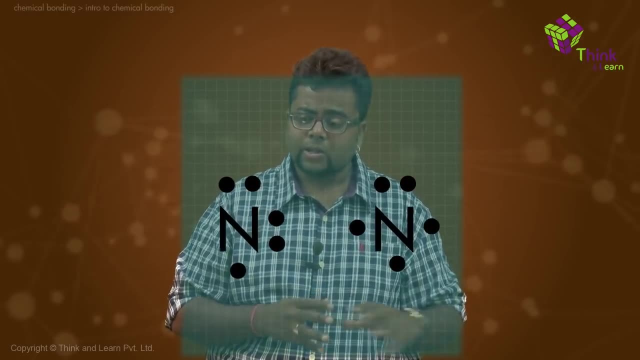 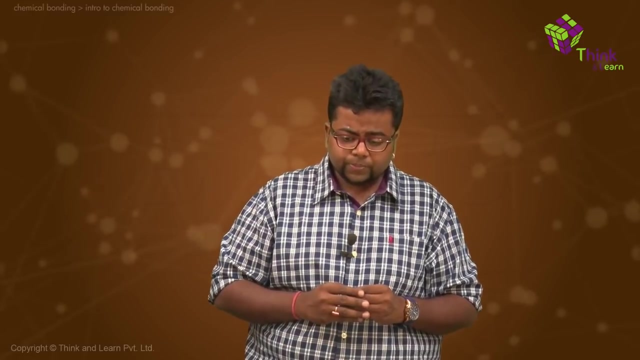 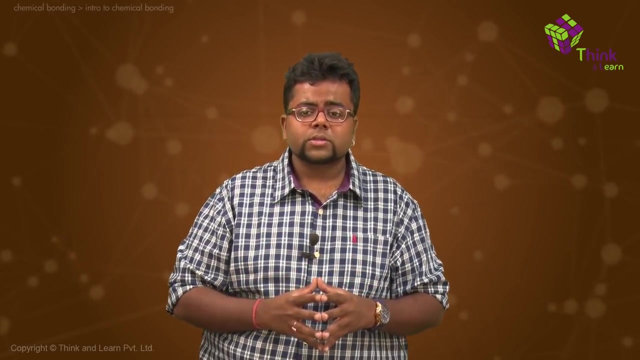 they are just trying to show it symmetrically because this structure can be used later on in a compound also. So if you draw any of these 2 structures, it is absolutely correct Now, when we as human beings fall into different surroundings. 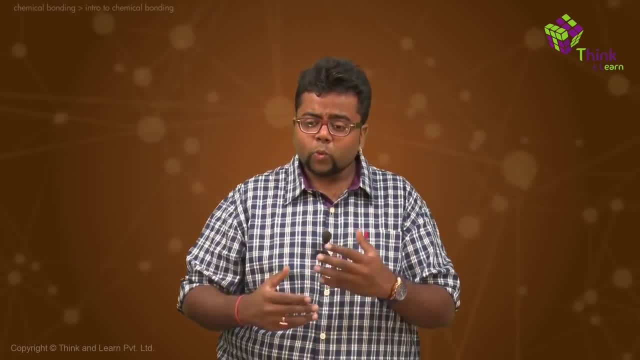 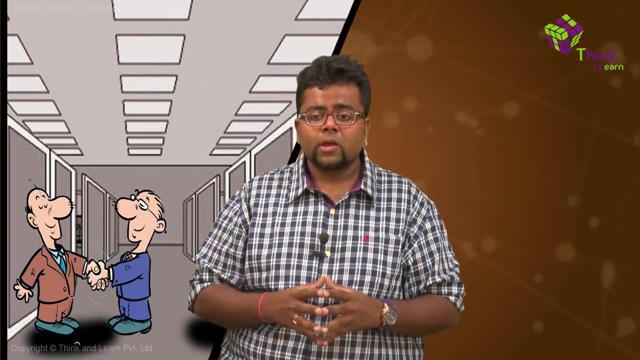 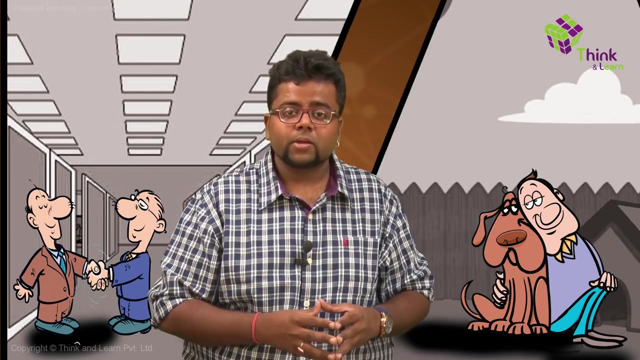 or we undergo different interactions. our way of bonding with the other person is different. If we are in a business meeting, we have a formal interaction. If we are with our own pet, the interaction changes completely. If I am with my mother,